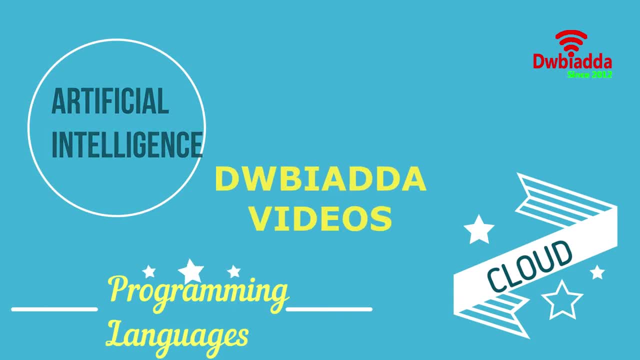 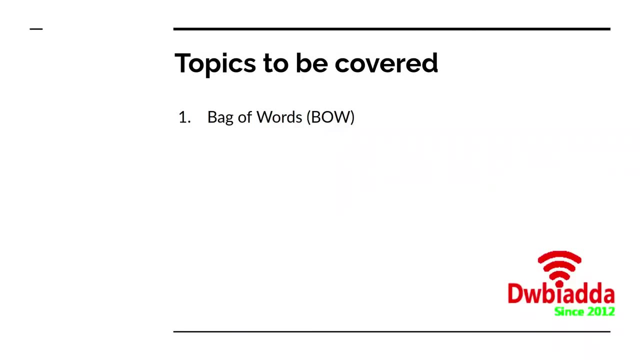 Hello everyone, welcome back to the lectures on Natural Language Processing. In the last lectures we have seen the three building blocks of NLP, ie Tokenization, Stemming and Stop Words Remover. I absolutely hope that you are comfortable with the concepts and you. 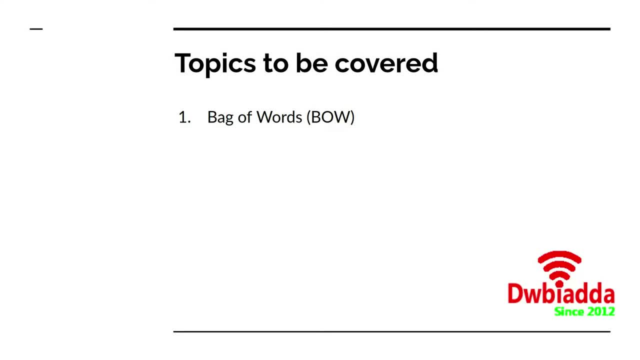 have practiced them enough so as to get comfortable. Today we will be starting with a new topic, which is known as Backup Words or BOW. So the first thing that should come in our mind is that what exactly are Backup Words and where it is used? So what happens is that. 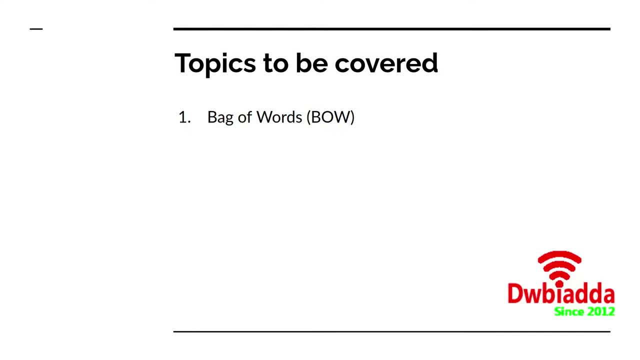 typical machine learning algorithms actually takes numericals as input. The input format is always in the form of numericals, Like I have told you before as well, whether you like, consider the case of logistic regression, SVM, NIV, bias or artificial media network as well. They take numbers, numbers as in the input. 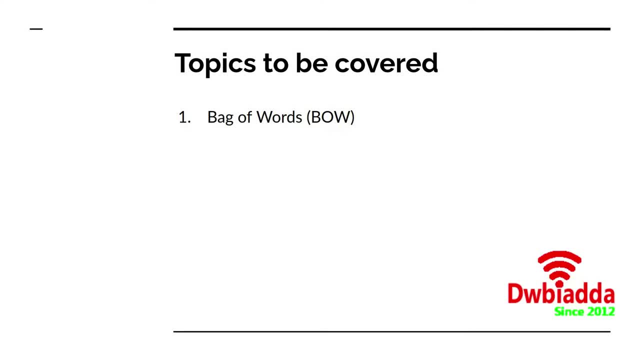 But we are actually working with text, So there must be a way so as to convert this text into the numerical format so that we could give them as an input to our machine learning models and get the desired output. So Backup Words is like one of the methods. 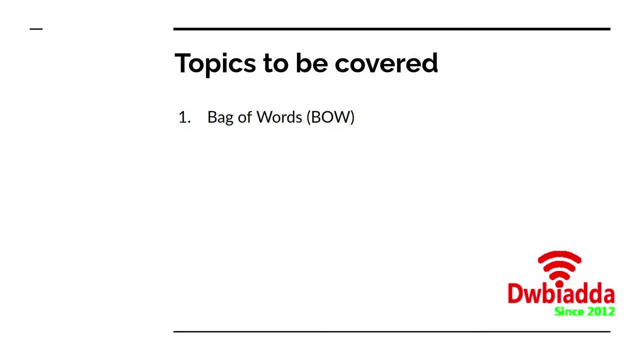 that is used for the same. So as of the name, it is very clear that we have a bag and in that bag we will actually put in all of the words Like there does not exist any bag physically, but let's suppose in the memory of the computer there is a bag and we will actually put all 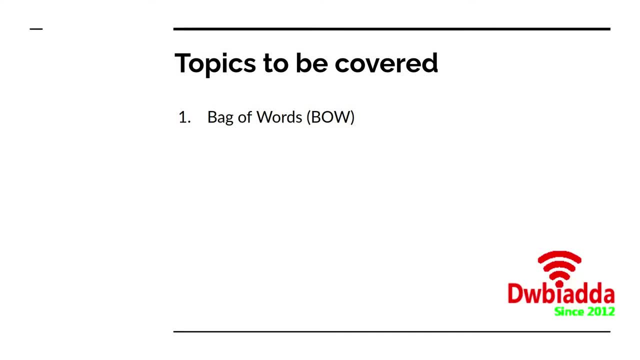 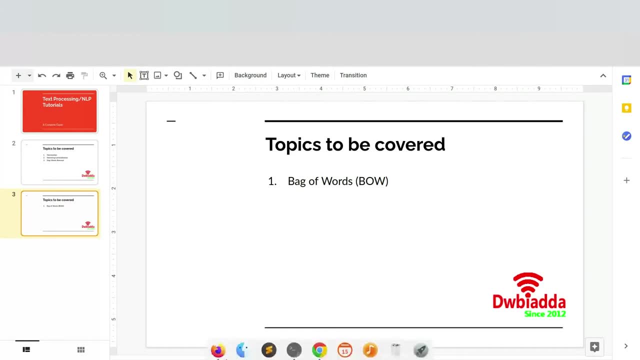 of the words that appear in the text in that bag Right. So I will explain more about Backup Words like: while we are doing the practical. So, without wasting much of our time on this, let's get started. I will quickly go up and fire my Jupyter notebook and, as you can see, 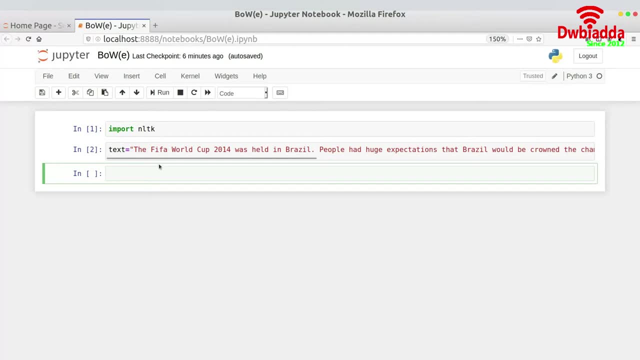 I have already imported some of the required libraries and I also have given one text, which is the FIFA World Cup 2014 was held in Brazil. People had huge expectations that Brazil would be crowned the champions. However, they were thrashed badly in the semi-finals and eventually 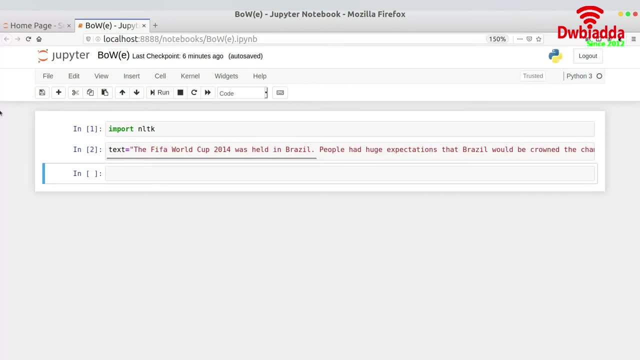 finished in the 13th. So this is the text I have, and now I want to create a Backup Words model using it. Right, A Backup Words model. So in Backup Words model, what we will be doing is that we will be basically like counting the frequency of the words, Like, let's suppose, if the appears five times. 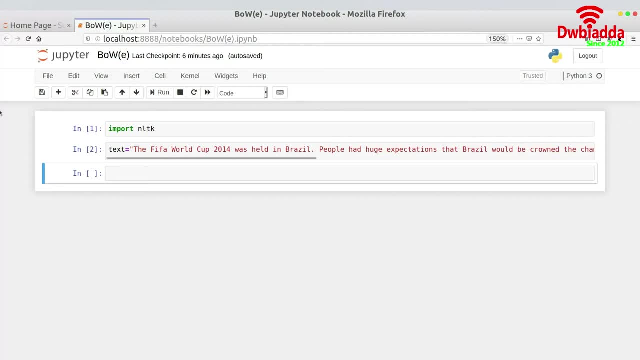 in this, like in this text, we will actually tell, okay, the is appearing five times. Like, if world appears seven times, we will actually tell okay, word is appearing seven times. and if world appears eight times, we will actually tell: okay, word is appearing seven times, and so on. Right, So let's just like, let's just do what I just doing. So, as you might have, 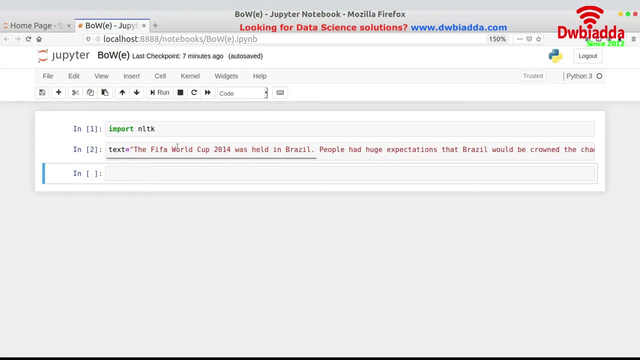 already guessed, we need to actually like a. we need to actually get all in all of the words right. We need to get all of the word and then we need to calculate the frequency So as to get the words. we will actually have to tokenize the sentence. but before tokenization, 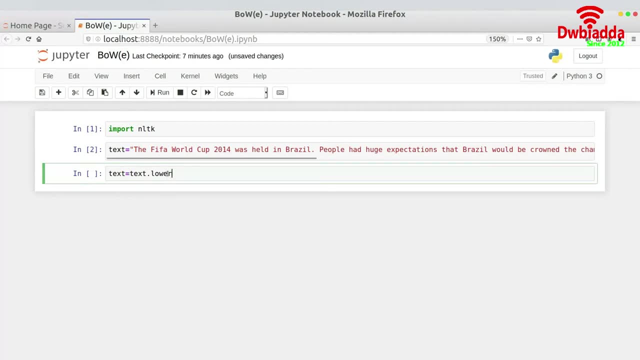 I would eventually convert this sentence into a lower form So as that the smaller letters and the capital letters do not differ like small than other, and the large there is not treated as like marked. So once I've converted this into a lower type of text, lower sentence, I will now extract: 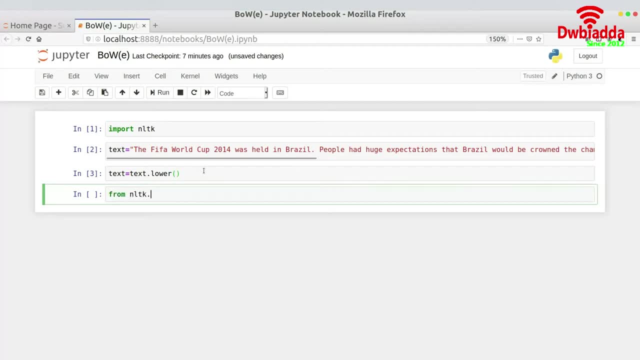 or import the tokenize sentence from nltktokenize import. I would be using the word tokenization, import word tokenize and then I would store the result in a list called result, which is basically word tokenize underscore text, and now you could basically see like how result looks like. and now what I need to do is that I need to like get in the frequency of all. 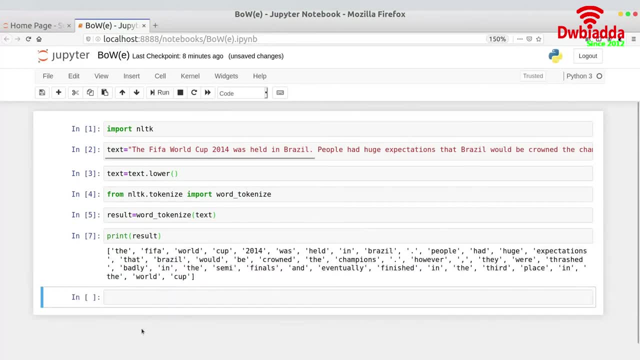 of the words that are present over here, like frequency of all of the words. Okay, so getting the frequency is very easy. I need to iterate over the list twice and print the frequency. So I would be doing the same. that is for before, like printing the frequency. let us 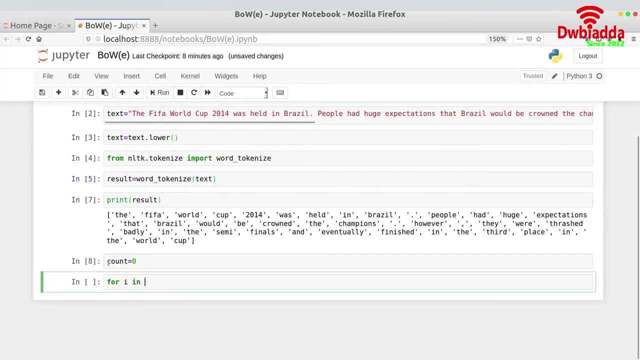 define a variable, let's say which is cow. So for i in range 0 comma len of list or len of result. for j in range 0 comma len of result. if result of i is equals, equals to result of j, then what we need to do is that: 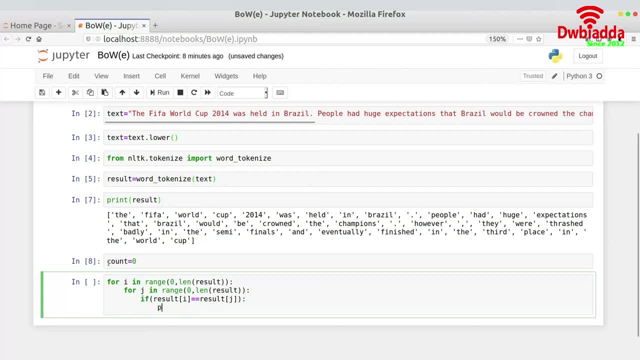 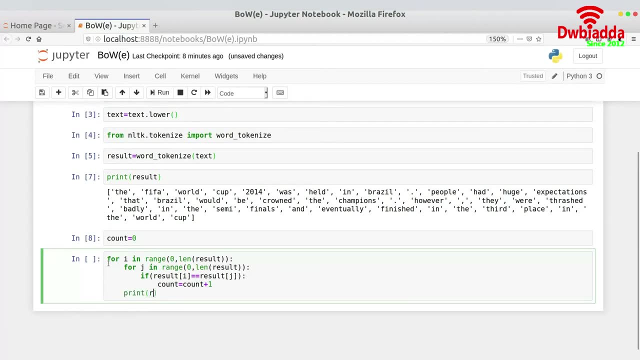 we need to print- sorry, we need to like increment the value of count, So count is equals to count, So count plus 1. and then what we need to do is that we need to print result comma count right, and then I would actually print something like count of 0, and it should be result of. 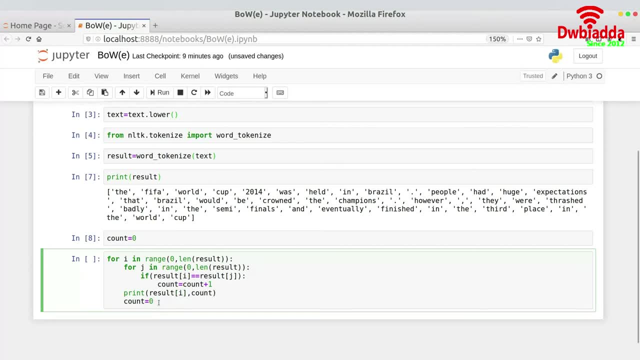 i comma count, basically, and then, like I will give, like, okay, count is 0.. So it will actually give me frequency of all of the words that are present in the whole text, right? So I will just run this piece of code for you. 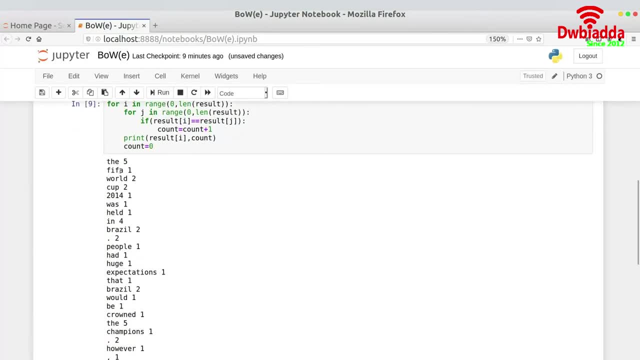 So, as you can see, like the appears 5 times, FIFA appears 1 times, world appear 2 times, was appear 1 times, held in appear 4 times, Brazil 2 times, full stop 2 times and all of that kind of stuff. So we have gotten the frequency over here. 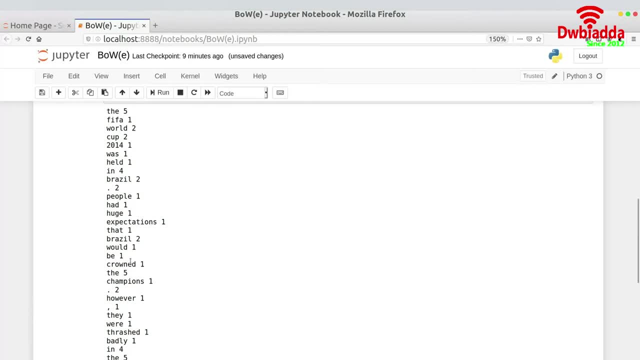 So, once we have gotten the frequency, what we need to do is that we need to put in all of these words in a back. but before putting in all of these words, just think that, like this is a very small sentence, right, we could have a text with millions and millions of. 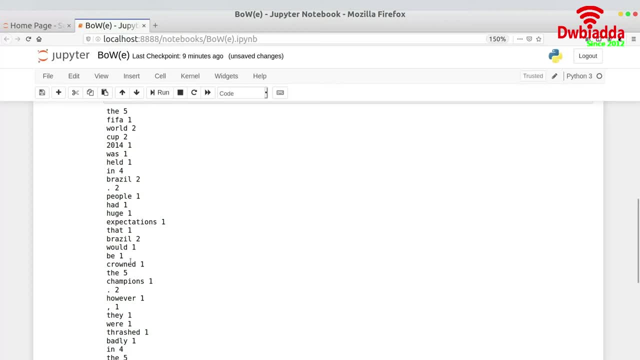 lines, millions and millions of lines, like as we generally do have in the real world cases of NLP. So what do you think it's like a good idea to actually put in all of the words in that back, because obviously the size of the back might be limited and we might not be able. 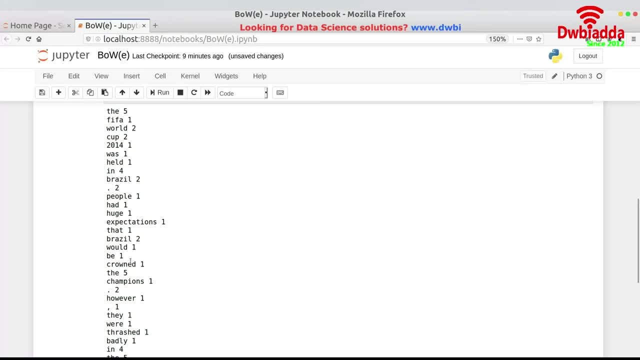 to put in all of these things. So, yes, if you are thinking that we need to put a cap and the words that we would be actually putting in the back, like cap, in the number, in the frequency of the words that we will be putting in the back, then absolutely you are right and this is what we do: a bag of 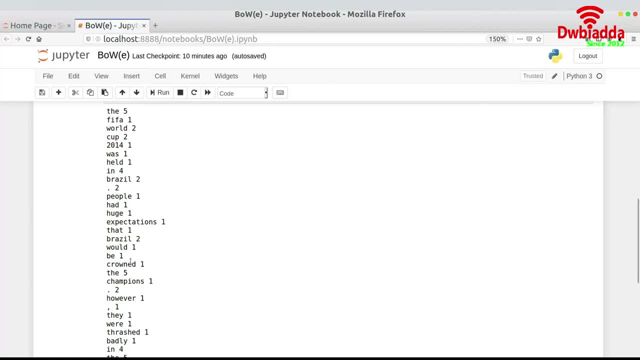 words. So what will be doing is that we would be like, like I would set up redefined Value. let's say that predefined value is basically two, or I guess two could be a good value over here. yeah, basically, let's say, if I like, have a predefined value, as I will only 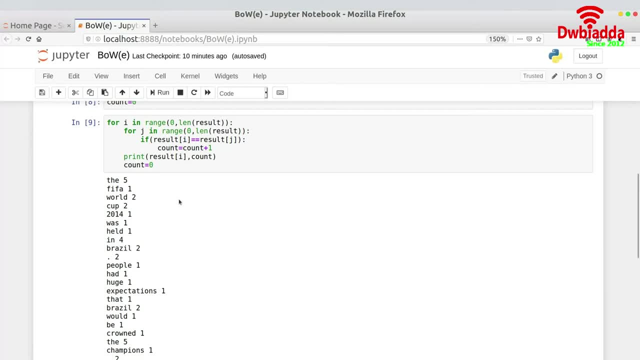 put in the words which has a frequency of greater than equals to two in my back. so this will actually reduce all of the computation powers and, based upon the words that will be receiving, we will actually like make a vector out of it. don't worry, I will explain. 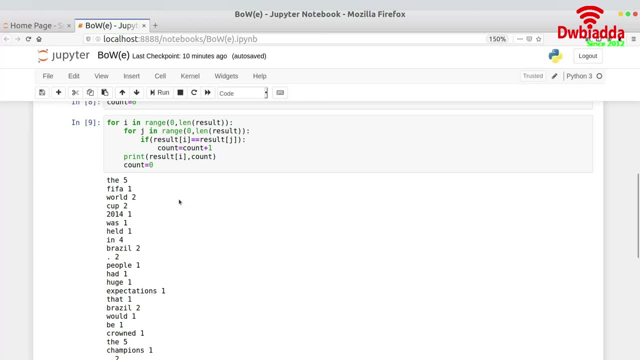 you what a vector is and how, like, completely like how bag of words exactly works. but as this point in time we are more interested in getting all of the words which have a frequency greater than or equals to two, so I hope like this is a very simple programming concept.